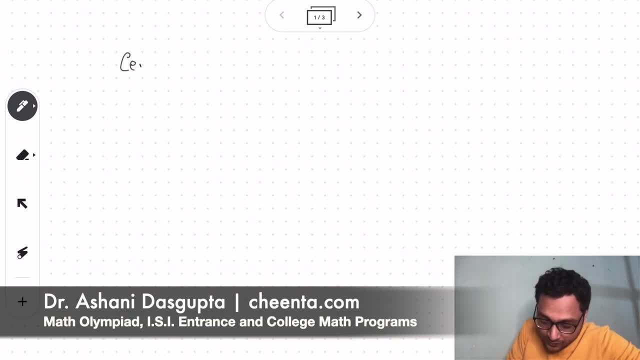 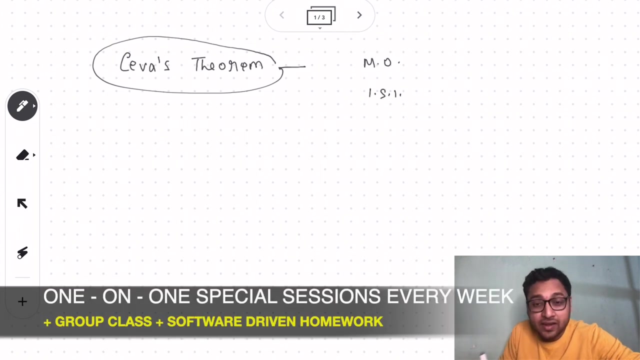 Okay, so today we will be learning about Shiva's theorem Now, if you have seen this theorem before, you will know how important it is to solve some of the most exciting geometry problems. Shiva's theorem is taught in the Math Olympiad program at Chinta. It is also taught in the ISI entrance and CMI entrance program at Chinta. 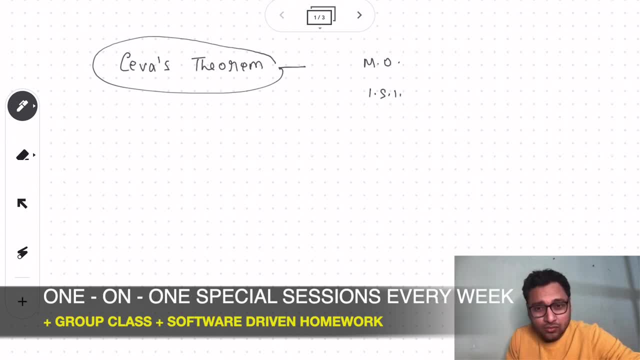 So what is this theorem all about? It tells us something about concurrent lines. So let me write that: Concurrent lines. What do I mean by concurrent lines? Well, if I have two lines which are not parallel to each other, those two lines will definitely intersect at a point. 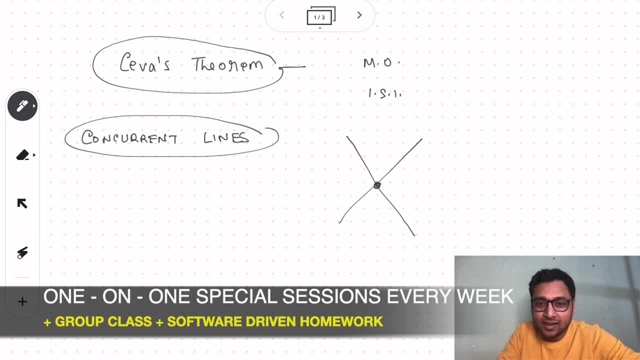 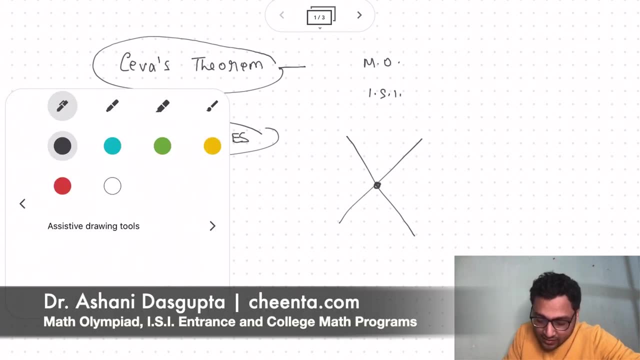 If they are not parallel to each other, of course. But what about a third line? What happens then? If I put a third line in this system, it may not pass through this particular point. So if all of these three lines passes through the same point, then we say that these three lines are concurrent. 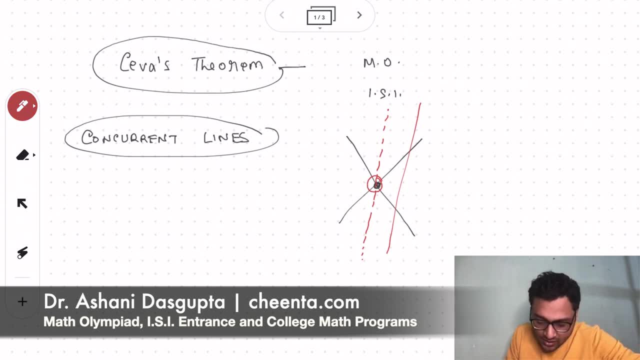 They pass through the same point. Similarly, if I have a fourth line which is passing through the same point, we say: these four lines are concurrent. So this is the meaning of concurrent lines. And what does Shiva's theorem give us? 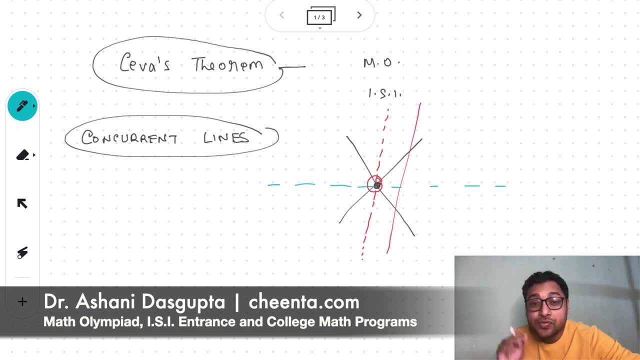 It gives us a condition when three lines in a particular triangle are concurrent. So to understand Shiva's theorem, we need to understand the following: To understand Shiva's theorem, we have to first understand the word Shavian. So let me write that down. Let's understand the word Shavian first. 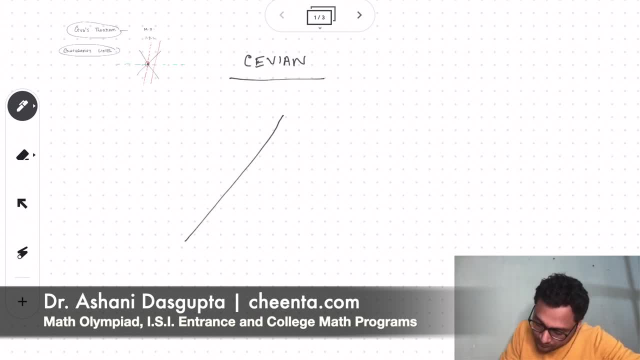 So what is Shavian? Well, you take a triangle. So I'm doing this in the context of a triangle, Let's say ABC. You start from a vertex and you join the vertex. You start from a vertex and you join the vertex. 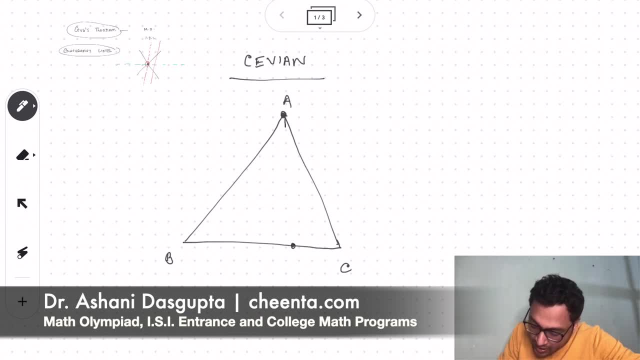 You start from a vertex and you join the vertex And you join a point on the opposite side of that vertex. So maybe this is P Any point, Any point on the opposite side of that vertex. So AP, this particular line is a Shavian. 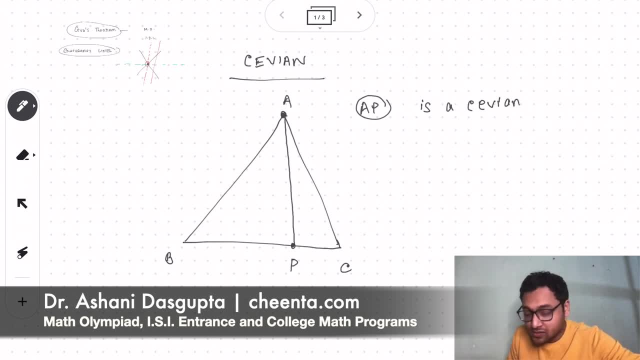 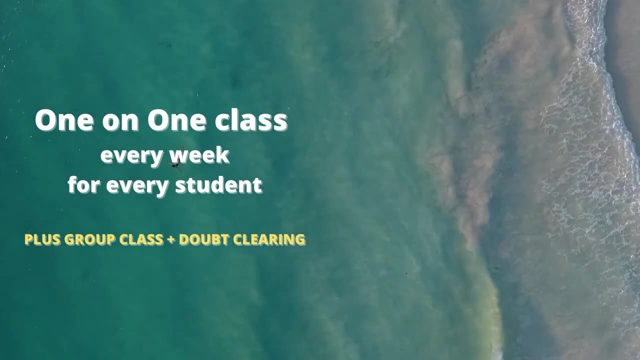 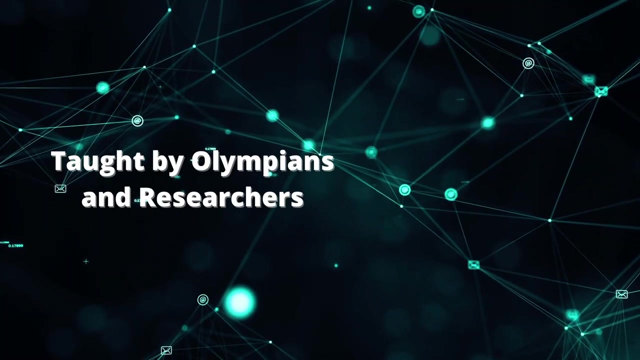 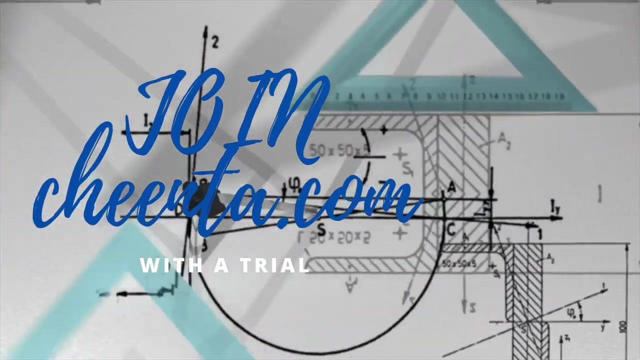 That's how we denote it. So, for example, median is a Shavian Shavian, That's how we denote it. That's a special Shavian, So we use it in aelling of aбoumувlэ. So we use it in aelling of a boumufly And we'll take this information here, And we'll take this information here, And we'll take this information here. So for angle by sector, angle is also a also a Shavian. 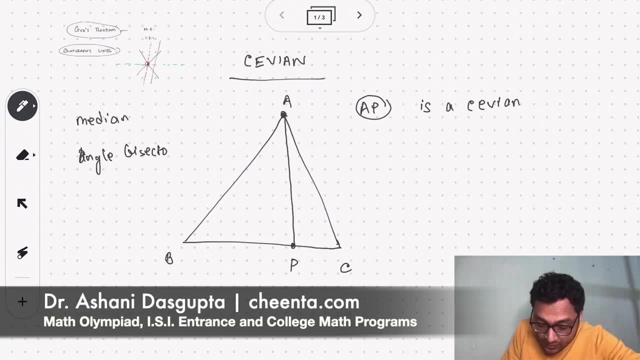 So, in terms of angle and square, angle is a square, Is also a square, Is also a Sói L andÆ, where angle is expired is a stated sugge L andÆ. so that means that angle beingается, or an angle that is also a sentient. 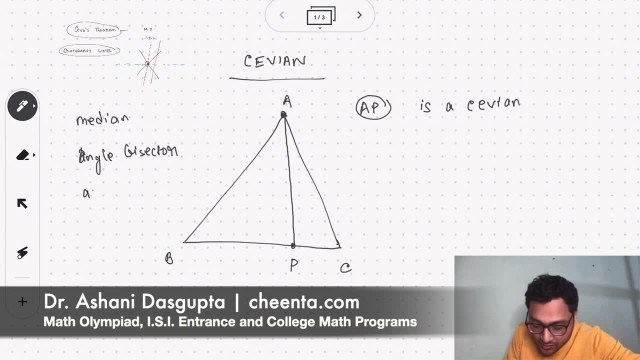 Similarly, altitude is a chevion. So we have all sorts of special examples of a chevion. So these are special examples And the chevion is the general term we reserve for all such lines. OK, so we understand what is a chevion, now Great. 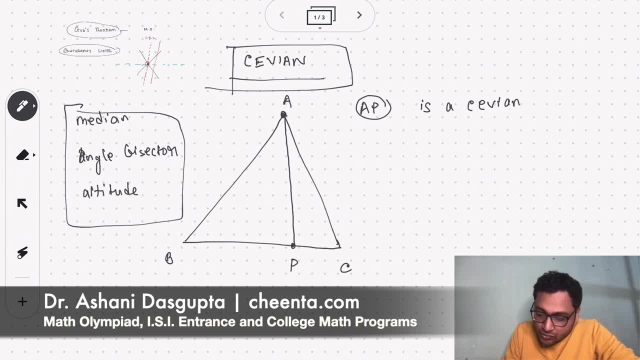 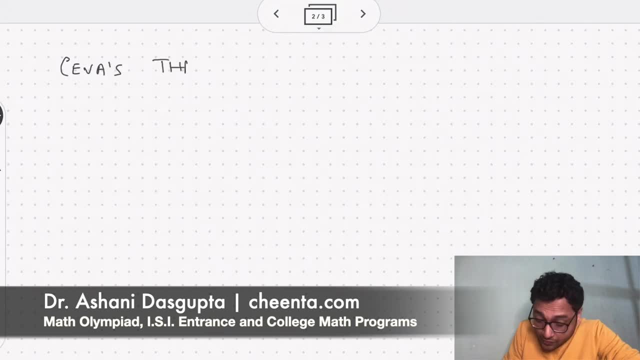 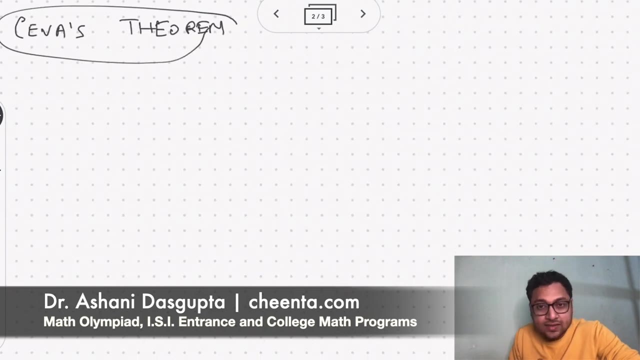 So when we will now talk about the statement of the Chever's theorem, So here is the Chever's theorem. We often use the converse of the Chever's theorem instead of the Chever's theorem itself. So what is the statement? It says that if you have a triangle, ABC, any triangle. 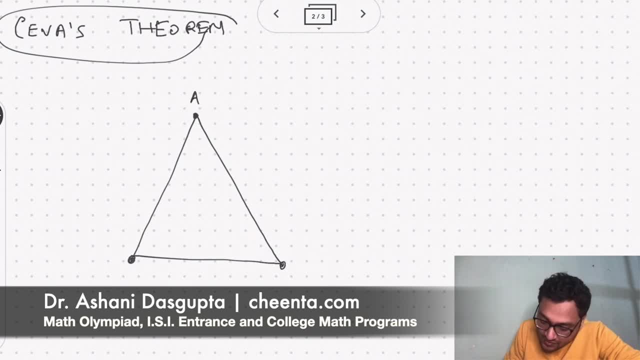 ABC. And if there are three concurrent chevions, So one, Two And three. So if there are, if there are three concurrent chevions, Let's say the feet of them are D, E and F, Then a particular ratio is true. 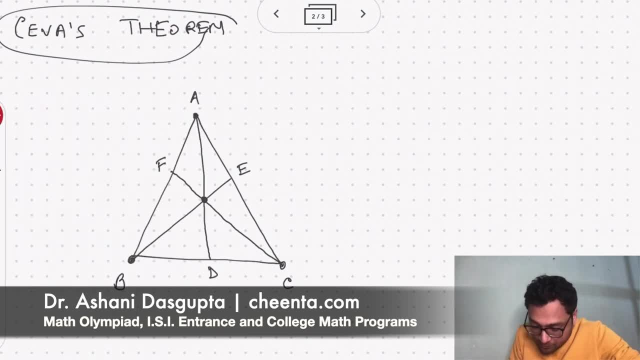 So what ratio is that? Well, you start from B. OK, I'll tell you how I remembered this. OK, so you start from start from any vertex. Let's start from B, B to D, D to C. So I write BD by DC times: C to E, E to A. 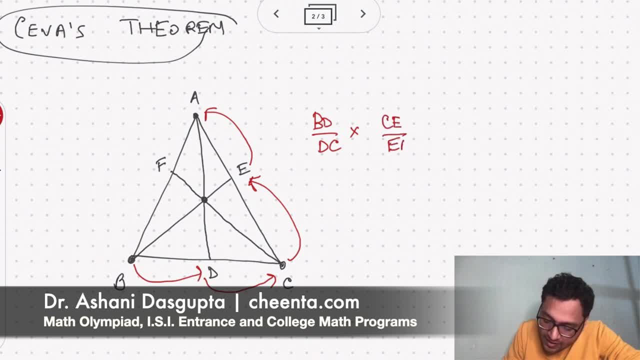 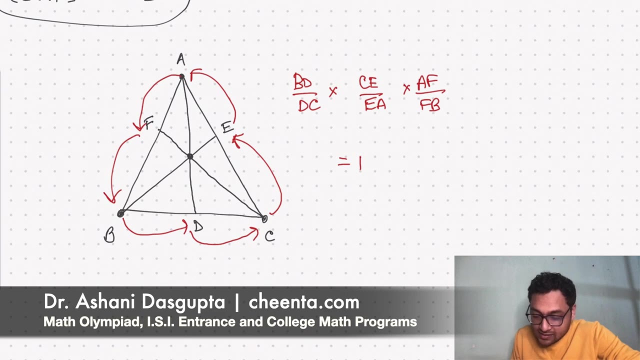 So I write CE by EA, And then A to F, F to B, So I write AF by FB. This is equal to one. OK, so this is the statement of Chever's theorem. So it says that if AD BE CF, 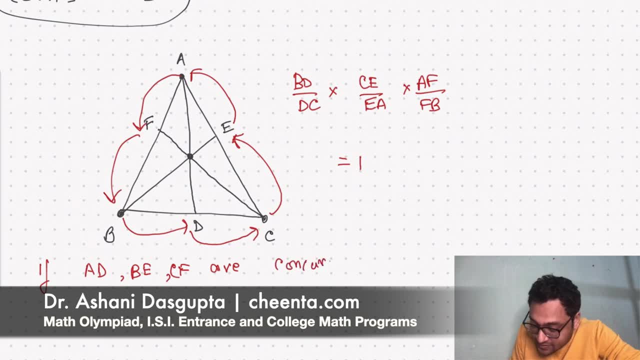 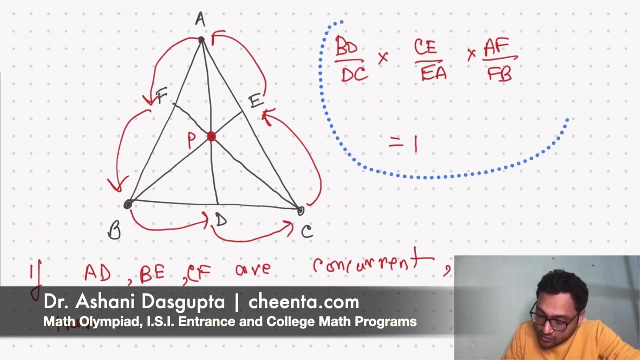 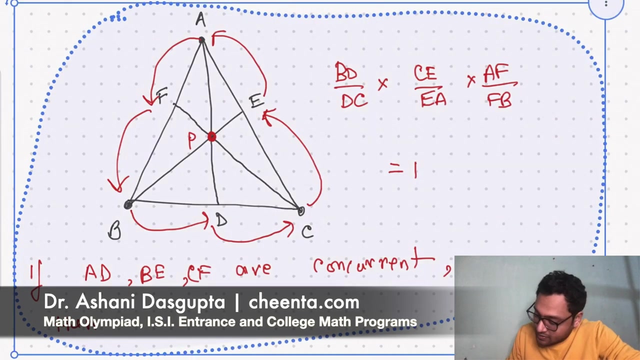 Are concurrent, That is, they pass through the same point. Let's call this point P, Then We have this, Then we have this particular Condition. Maybe I can just make this a little bit smaller. OK, And let's put this here. 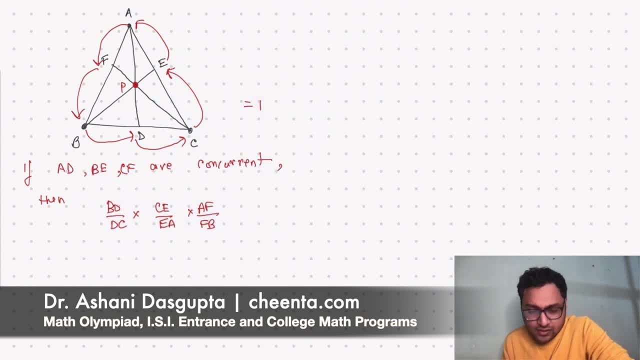 Then we have this condition. So how are we going to prove this thing? Because this is one of the most important theorems that you will face in math Olympiad training and in geometry per se. So how are we going to prove this? 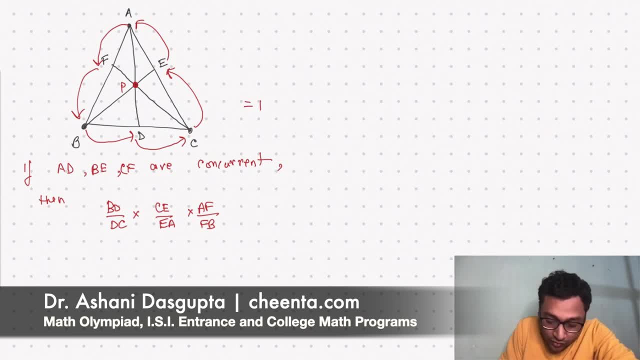 Well, we will be using the method of areas. So, the method Of Area. So what do I mean by that? Well, I'll give you the first step, Step one. And the step one is: You take This area. 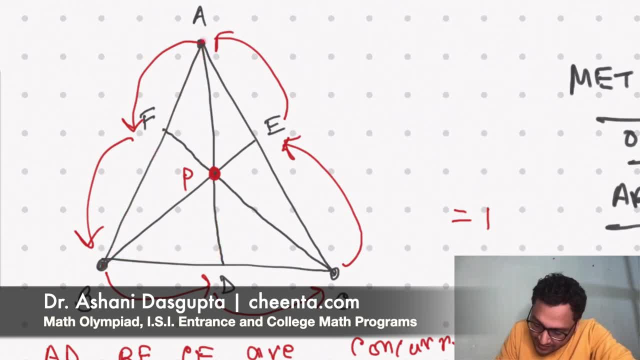 ABD And you take ACD, You take their ratio. So ABD And ACD, The ratio of these two areas, This is Equal to BD over DC. Why is that? Because this is a very powerful result. 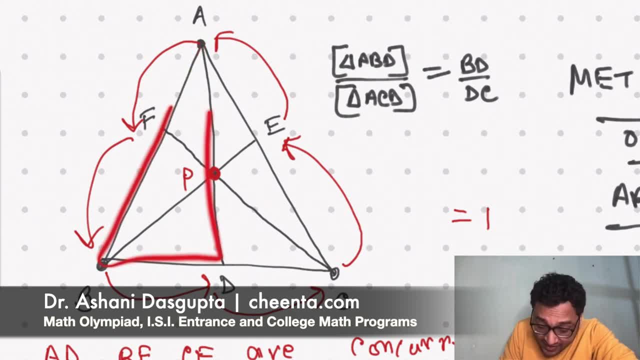 Simple but powerful result. If the vertices of two triangles are same And if their bases are on the same straight line, Then the ratio of the areas of these two triangles Is equal to the ratio of the bases. We discuss this at length. 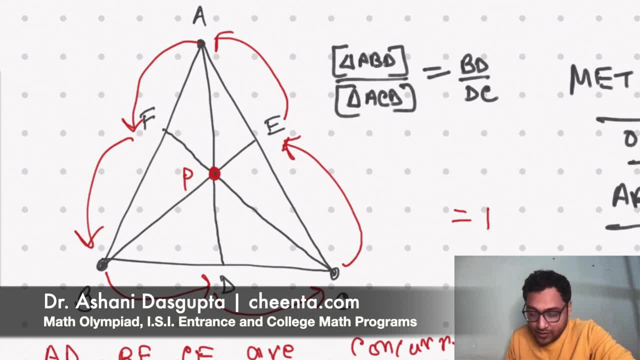 In other videos And as well as in our Math Olympiad program. It's a very important tool in geometry. Ratio of the bases Would be equal to the ratio of the Areas of the triangle. Why is that? Well, if you drop a perpendicular, 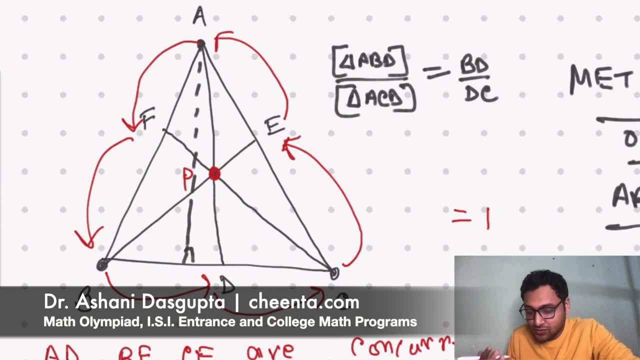 Both of the triangles will have the same height. So the If you take the ratio of the areas, The heights will cancel off. Half will cancel off. Only the ratio of the bases will remain Okay. So now that we understand this, 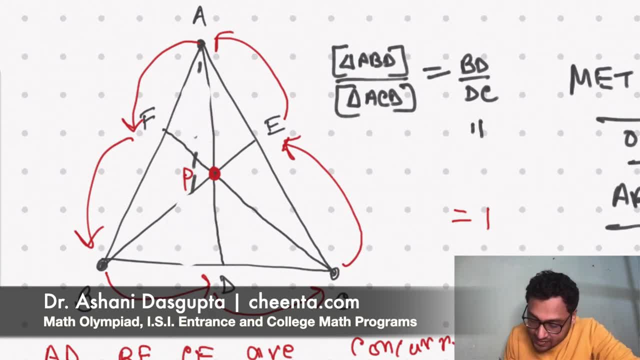 We can also say That this BD by DC Is equal to Triangle PBD By triangle PCD, The ratio of these two areas. So the ratio of these two Is also BD by DC, The ratio of PBD and PCD. 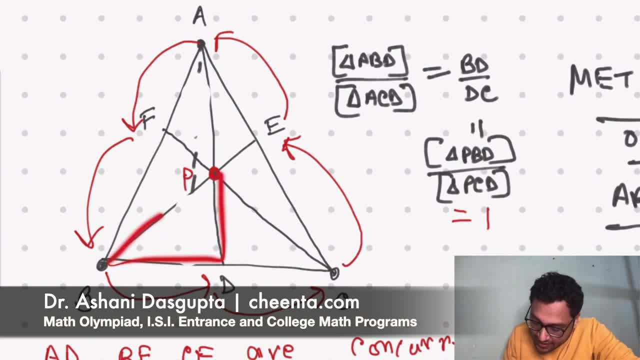 Is also BD by DC, PBD And PCD. So the ratio of the PBD and PCD Is also BD by DC. The same reason: P is the vertex. Both of them share the same vertex And the bases are on the. 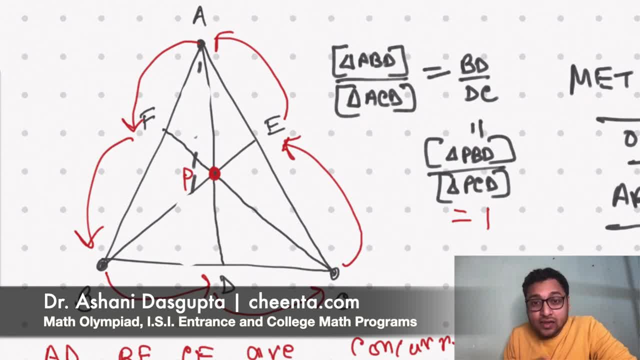 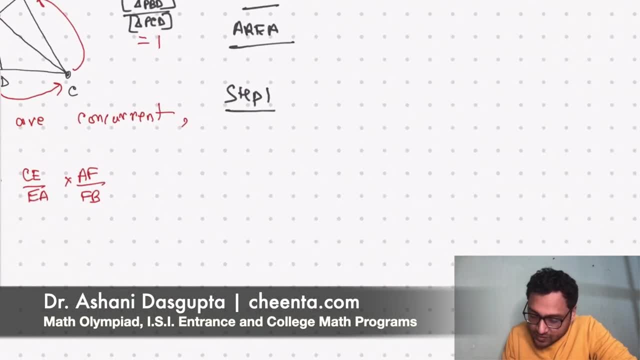 Same straight line. So now we will do a trick. The trick is called Subtrahendo, So I'll take, I'll make a little bit space And I will write that down. Maybe I'll Write the spelling wrong. 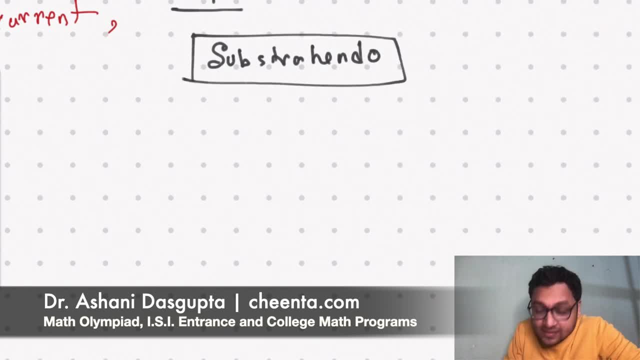 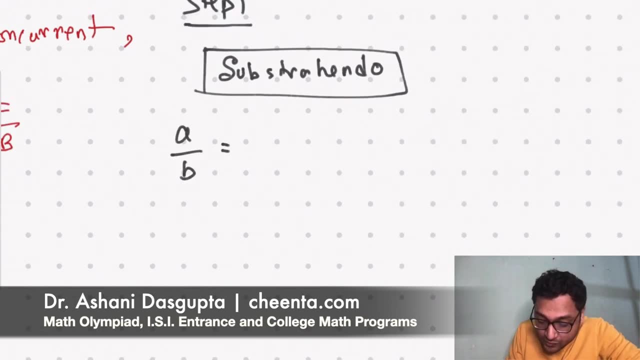 So What is this? What is this Tool of proportionality? Well, If you have A by B Equal to C by D, Then both of these ratios Will be equal to A minus C By B minus D. 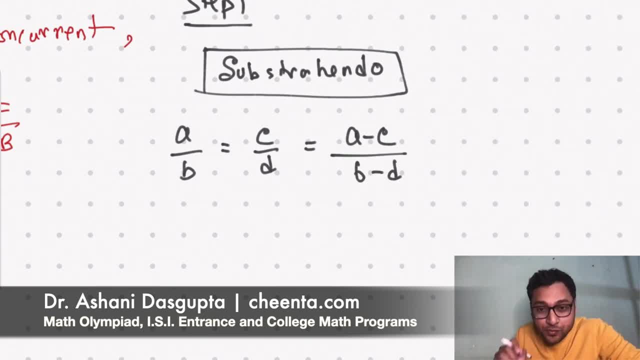 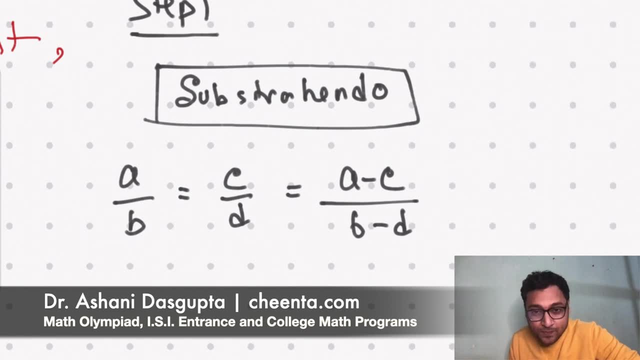 Why? Well, You can try to prove this And comment. Put a comment in the description With how you can show this To be true. It's very simple, But give it a try. Okay, Do this And put a comment. 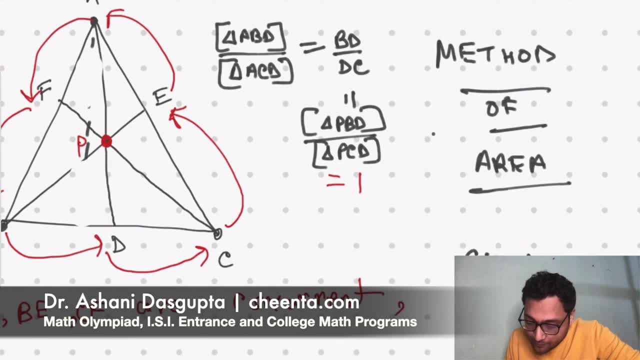 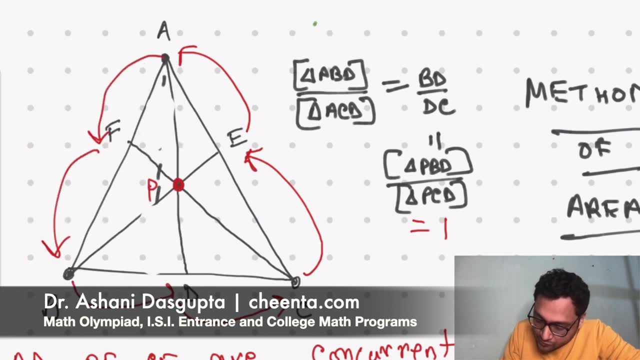 Let me see How you can do this. Okay, So we will apply this here. So we will Do This simple step Where we do A B D Minus P B D Divided by A C D. 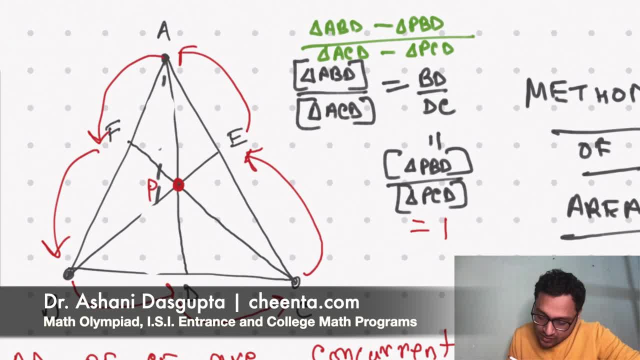 Minus P C D. So A B D Minus P B D Is Equal to This A P B Triangle And you can check that A B D Minus P B T, This big triangle. 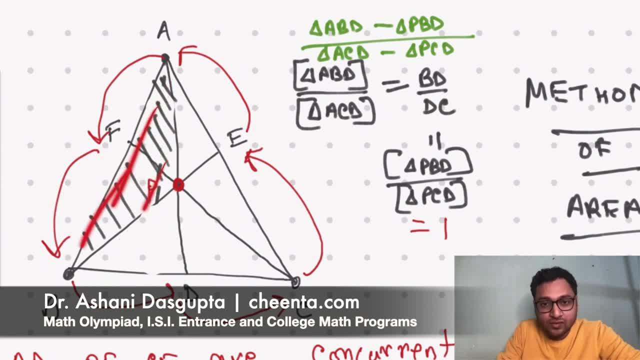 Minus The smaller one Is this Shaded one Right, And similarly This one will be A P C, A C D. Minus P C, D Will be A P C. So this is P. 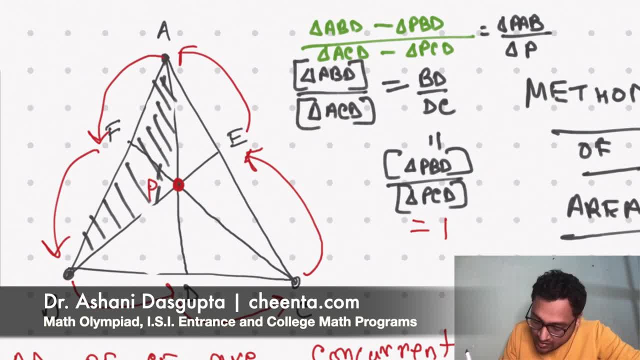 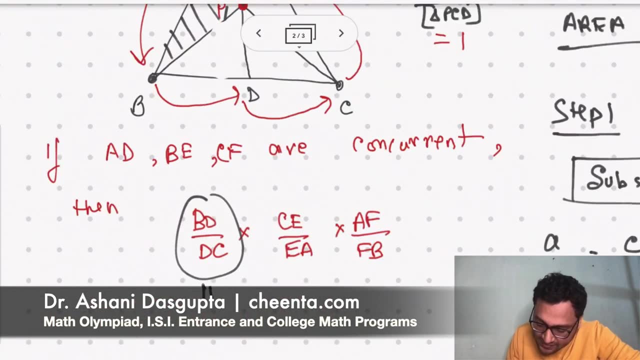 D By P A C. That is what B D By D C Is. B D By D C Is P A, B By P A C. That's what we got, Okay. 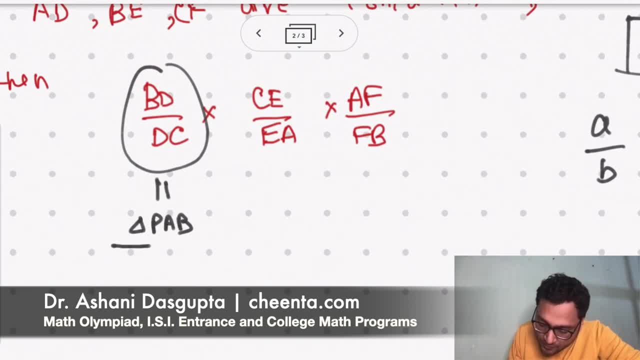 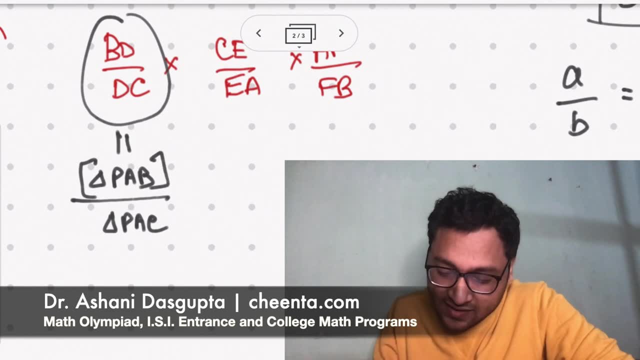 So B D By D, C. Right here Is Triangle: P A B, P A B By D. Similarly C E Over E A And A F Over F P Use. 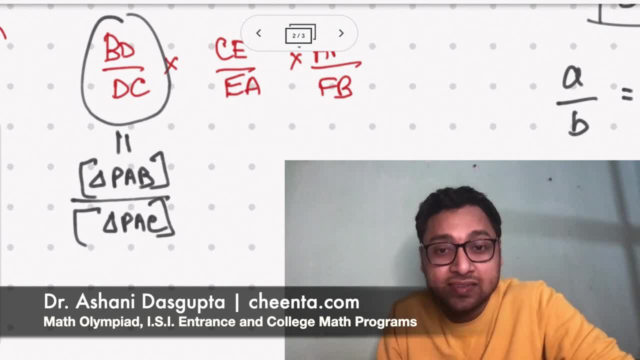 The Same Sort Of Strategy, And Then Check What Happens. If You Multiply These Out. Each Of These Ratios Will Be Equal To One, That's. 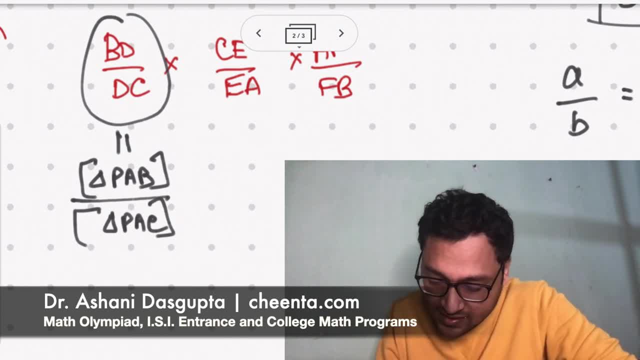 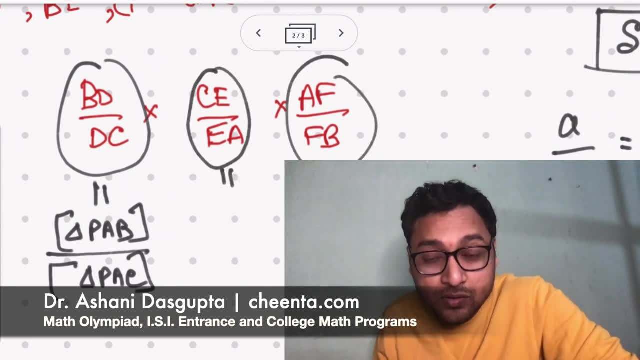 Our Goal. That's What We Tried. One To Prove This. If You Come Back To The Statement, You Will See That This Product Is You. 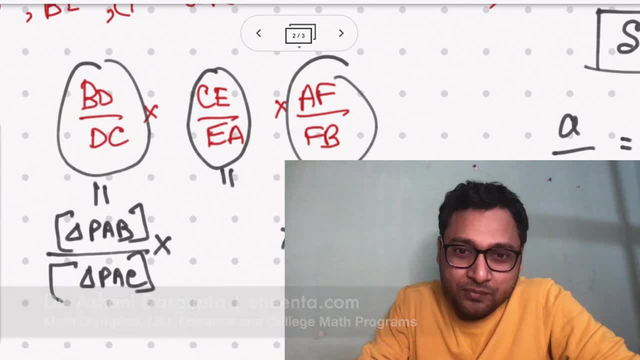 Keep On Doing Great Mathematics. I'll Come Back In The Next One. Okay, Bye.